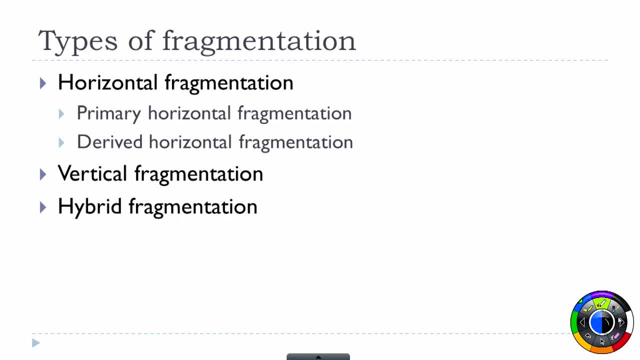 Vertical fragmentation is about vertically, with respect to the columns that are part of the single table. So we are going to break that is decomposed into multiple relations with respect to the number of attributes present here. And final one, the hybrid fragmentation is about the combination of these two. So 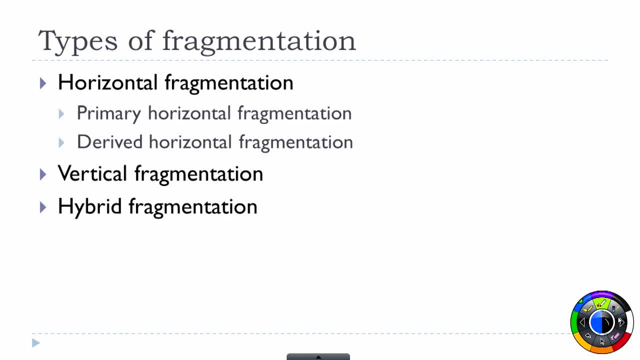 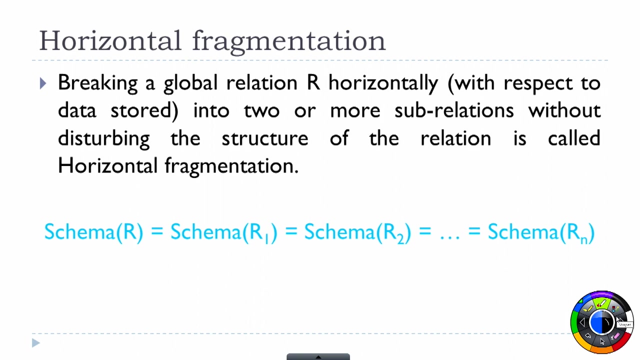 we take a table, we horizontally fragment this table and then we can fragment vertically the horizontal fragments, or we can vertically fragment the table and further. the vertically fragmented table may be horizontally fragmented further. So these two things are called hybrid fragmentation. So horizontal fragmentation is about breaking a global relation or horizontally into two. 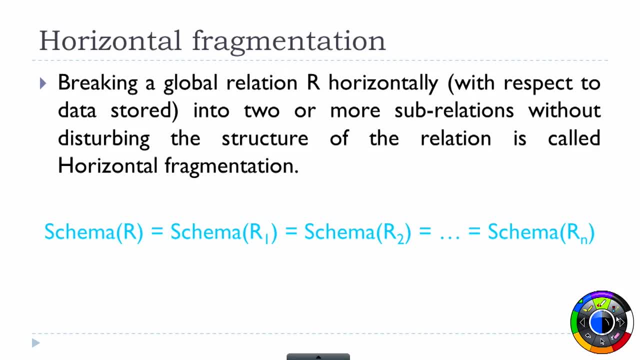 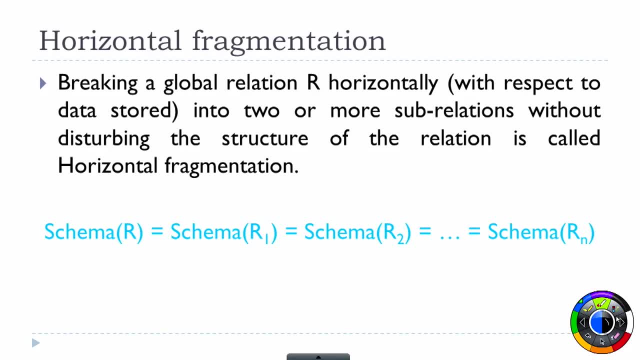 records: n records in a table, So some records may be placed in one particular site, some other record placed in different site, and so on. So we are going to horizontally fragment with respect to the data stored into two or more sub relations. So there is no change. 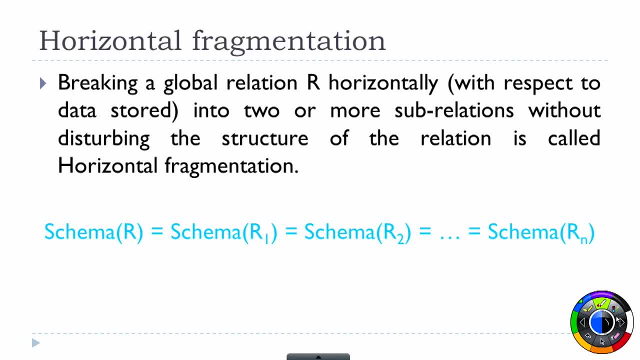 we do not touch the structure of the table. structure of the table is going to be same. So in such case, what we result is the schema for original relation and the schema for fragment 1, schema for fragment 2, and so on. all will be the same. That is what horizontal fragmentation. 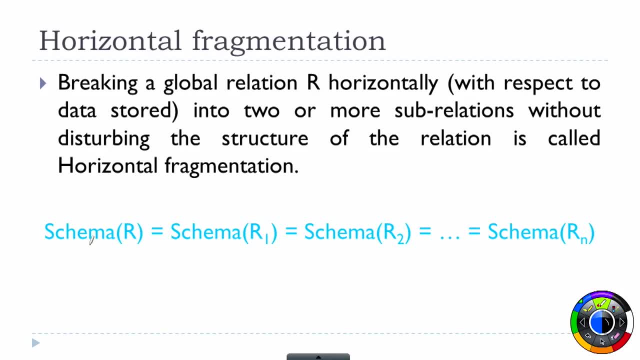 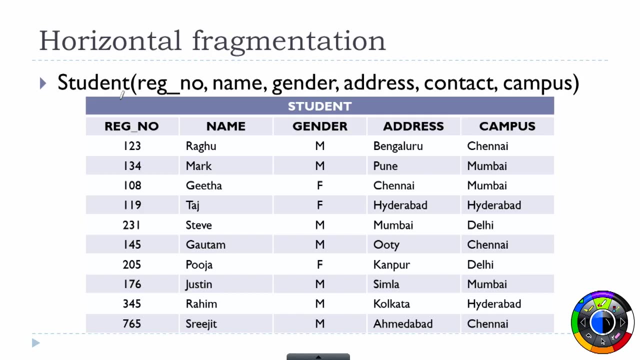 is about. We do not touch the columns, that is, structures. We take all columns. we include all columns in the result, but records are filtered. Take an example: Schema student is given with register number, name, gender, address and contact campus. Now we have many records in it. What I do is I am going to fragment. 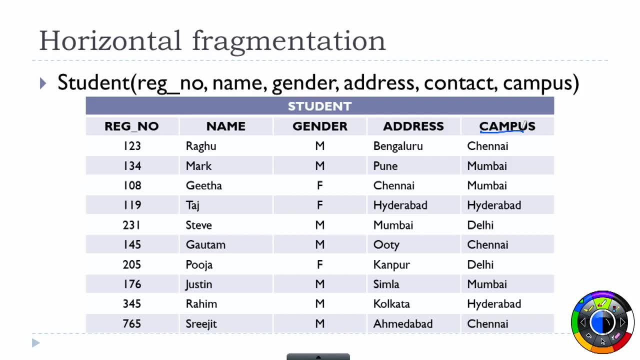 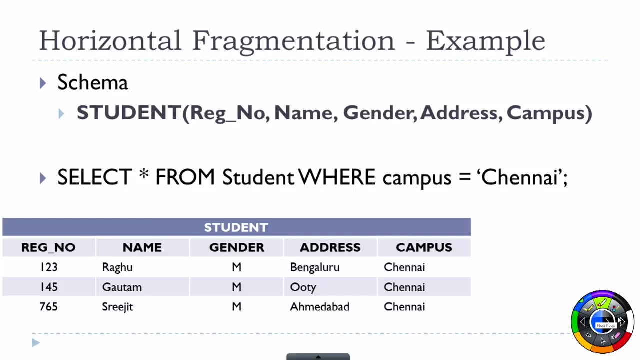 this relation based on the campus attribute, the values, the domain of campus attribute. I am going to choose to fragment this relation, So what I do is just simple: select condition, select query, select star from student where campus is equal to Chennai, that is, I put. 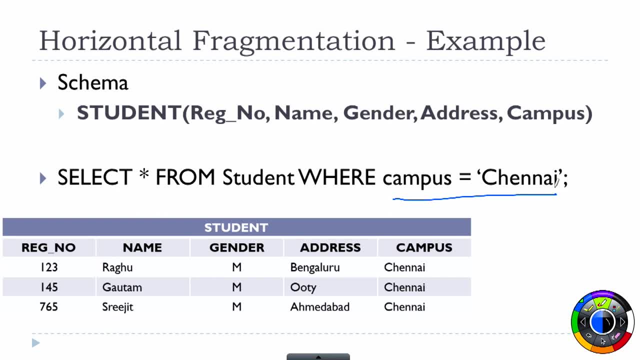 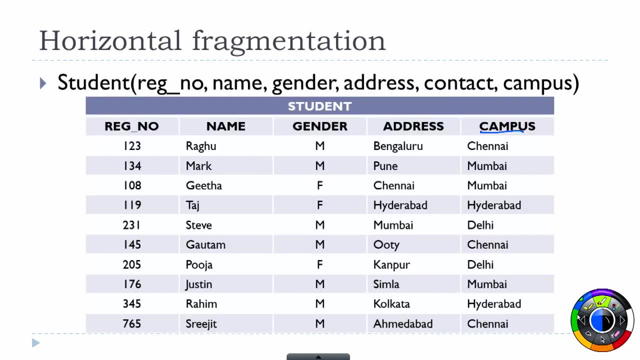 a condition, campus is equal to Chennai. That results in three records, These three records, these three records are from this original table. So this is one record. This is another occurrence of Chennai record. This is third occurrence of Chennai record. So it is very simple When I write a query like 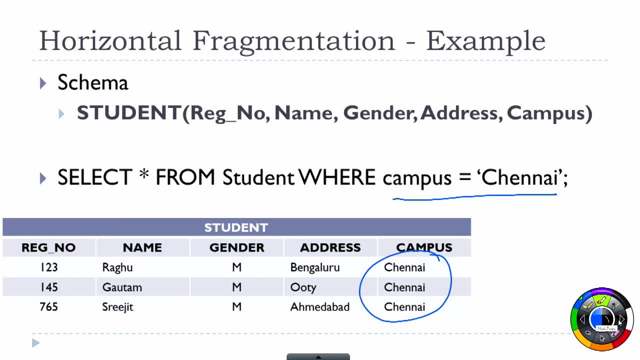 this. what will happen? It is going to filter the data and choose only those records from Chennai. So this is considered as one fragment. So, for example, I have campus record, So I have campus in four different locations in the country and all these students records. 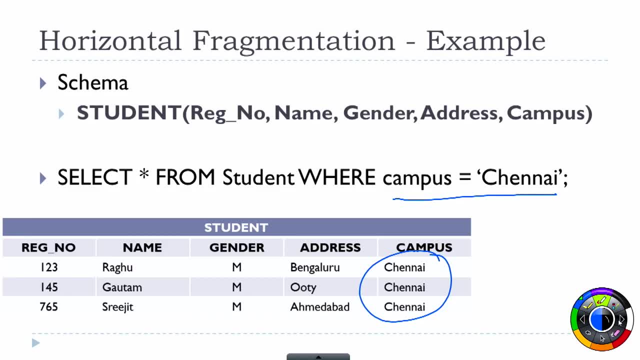 I want to store in each different locations. So Chennai students are stored in Chennai side, Calcutta- sorry Delhi students are stored in Delhi side, and so on. So this is another fragment. So select star from student where campus is equal to Mumbai. that is results. 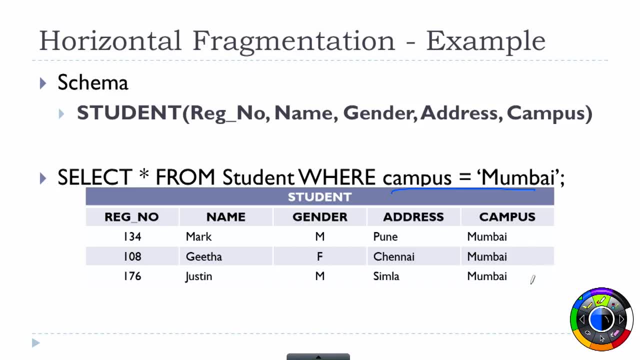 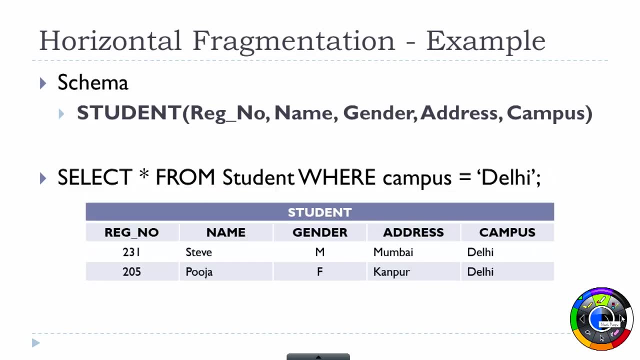 in another fragment where the campus value will be Mumbai 1D. So three records are taken from Mumbai side. So these records will be sent to Mumbai side. Another one campus is equal to Delhi. This will results in number of records from the student relation where campus is equal to. 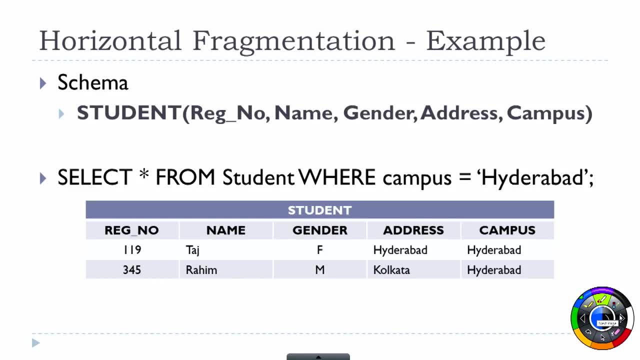 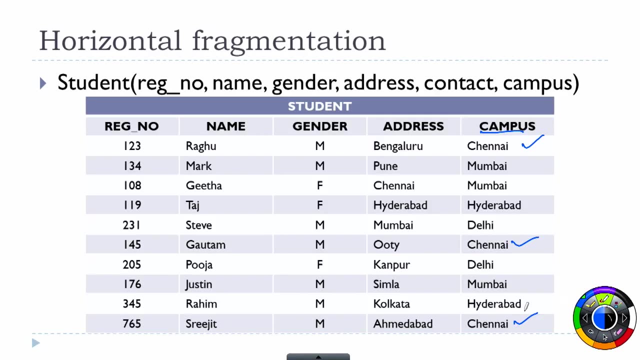 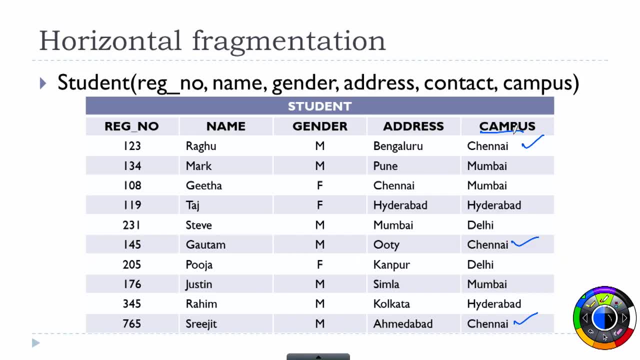 I have taken this original relation. from this original relation I have taken campus as the attribute. Where I am going to apply these conditions? Where Chennai is equal to, so campus equal to Chennai, we will get filter records according to the campus value. Then campus is equal to Mumbai- another Mumbai record, So I will get Hyderabad. 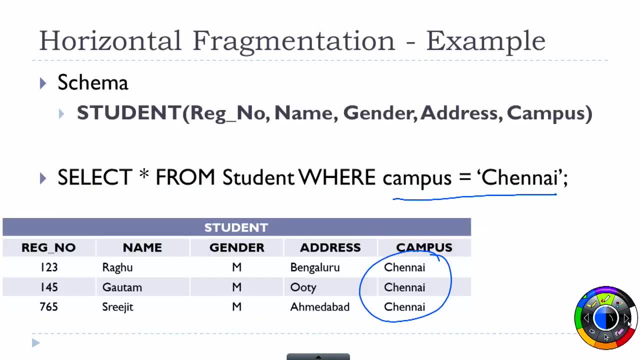 Hyderabad records. So all these records are going to be stored in different locations, into different fragments. So horizontal fragmentation is just as known as sub finite fragmentation. So instead of starting from the University, so we can start from the University Then. 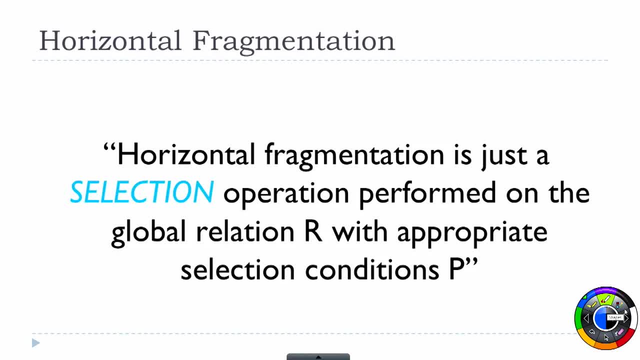 we go further, We will start from here. Similarly, the distance between pryzon options will be further. horizontal fragmentation is just a selection operation. what we do is just a selection operation is performed on the global relation R with appropriate selection conditions P. 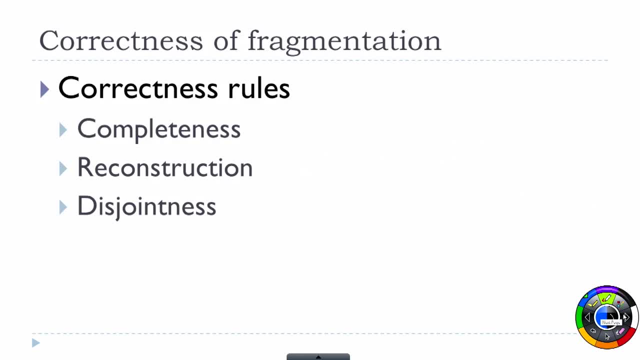 with appropriate selection conditions: P. Now the question is: are we doing the right thing? because it is not just as simple as what we are doing, what we have done so far for a student relation. So we have taken only one condition: where campus is equal to 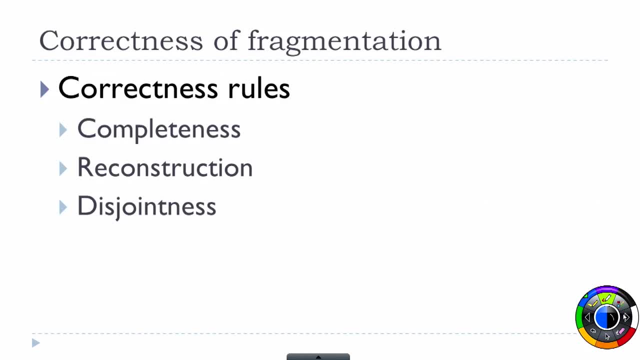 Chennai, but with different values. So the result is going to be a set of records, but is that the correct fragment? What we did is correct or not? So we have to verify that. So to verify that we have rules called three, rules called correctness, rules, correctness. 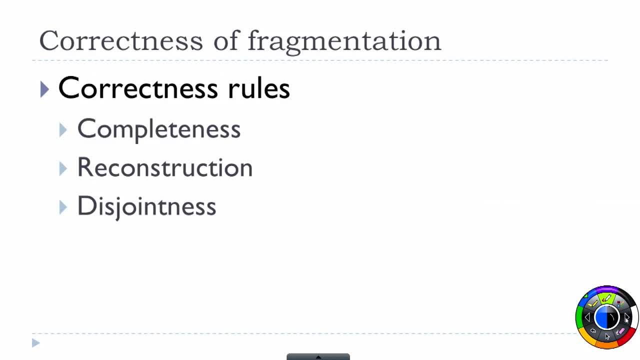 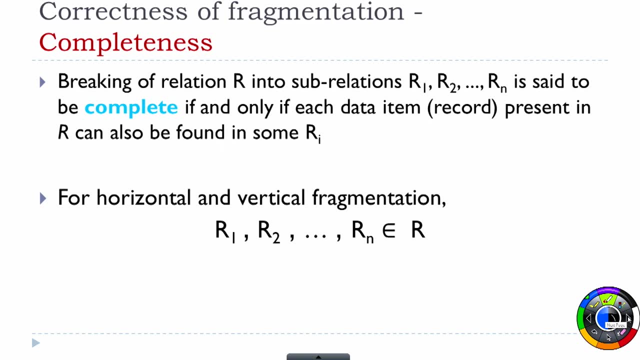 rules of fragmentation. So first rule is completeness, then reconstruction, then disjointness. So completeness is about Now: are these records present in some of the fragments or not, one of the fragments or not? So I have original relation R. that relation has 100 records within that. Now, 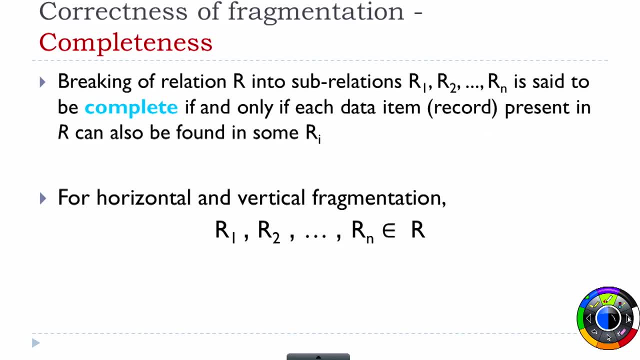 I fragment this original relation into 10 different fragments. Now what happens? Each fragment must have some record. each fragment must have some record. that means all the records in R must be fragmented into these sub-relations. I am not going to miss any data item. that is what the completeness is about, So breaking. 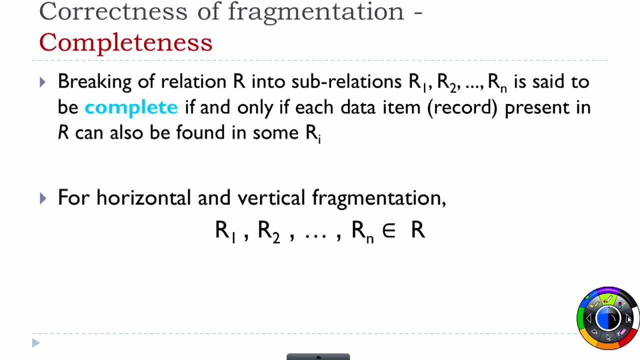 of relation into sub-relations is said to be complete if, and only if, each data item present in R can also be found in some R i. So what I say, what I say, is: the records of R 1, records of R 2, records of R n are all taken from R only are all taken from. 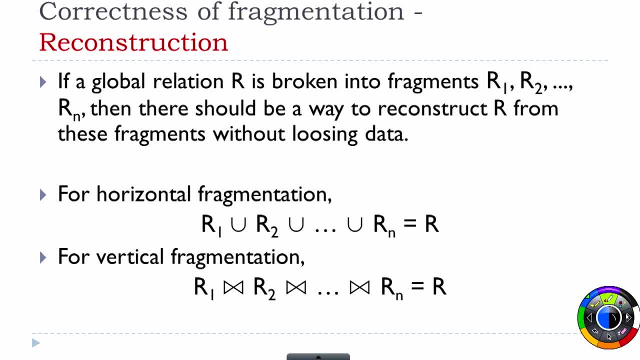 R only. So this is completeness rule. The second rule: reconstruction rule. if I fragmented my relation, broken my relation into different fragments, then there should be a way to reconstruct R from these fragments without losing data. So what I do, I have R, I have broken R into R 1 and R 2, and so 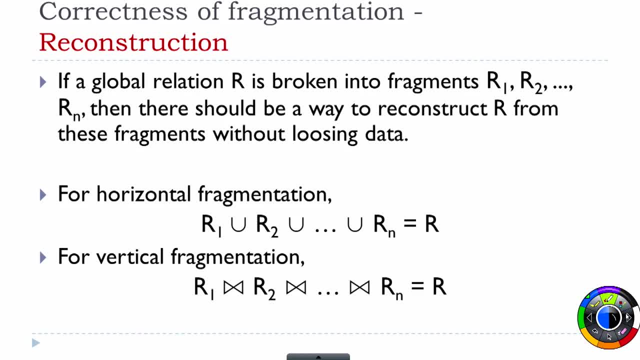 on some sub-relations. When I combine all these relations together, I am going to get my R back without any loss of information. That is the requirement. So the reconstruction is about. I perform some operation on the fragmented relation so that I am going to get back my R. So what I can do for horizontal fragmentation: 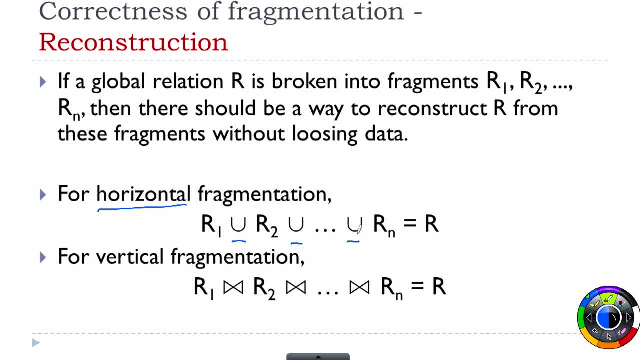 I can perform union operation, that union operation is going to get me the R back. So R 1, union R 2 and so on, all my sub-relations. if I perform union operation between all my sub-relations, I am going to get my back, get my R. 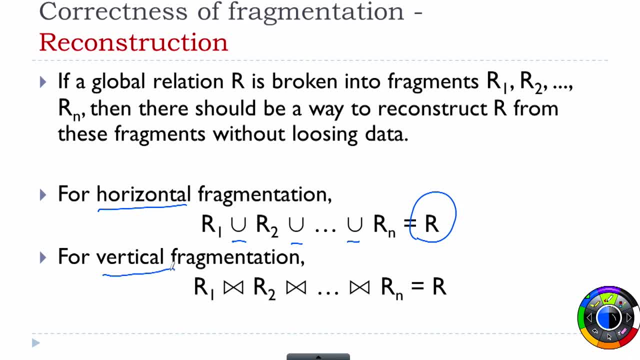 R back For. likewise for vertical fragmentation. I need an operation. Here. the operation is natural joint. So because vertical fragmentation, we are going to fragment the tables vertically with respect to columns. So in such case I need R1, natural joint, R2, natural joint. 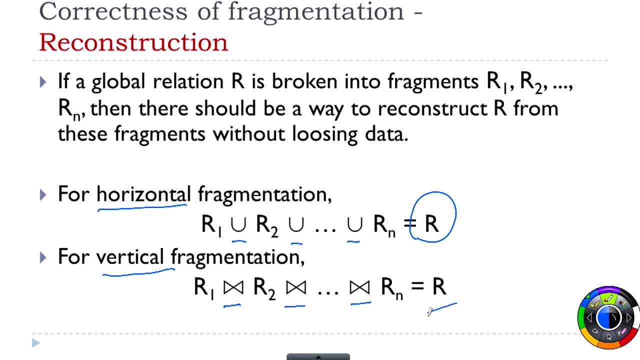 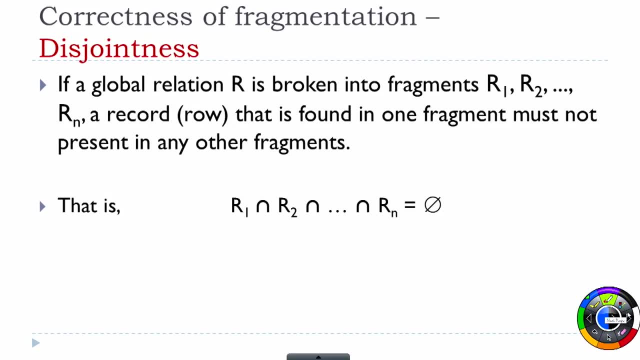 and so on. All the sub relations have to get me R back without any lose, any loss of information. So this is what reconstruction rule is all about. The third rule is disjointness rule. If a global relation is broken into fragments, a record that is found in one fragment must. 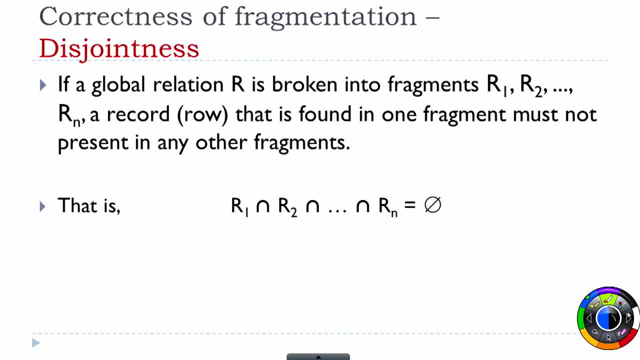 not present in any other fragments. So that is a one record which presents in R1 and also R2 will lead to redundancy. So redundancy is a important thing which has to be avoided in storing in the handling databases. So that is what this property is in R1. 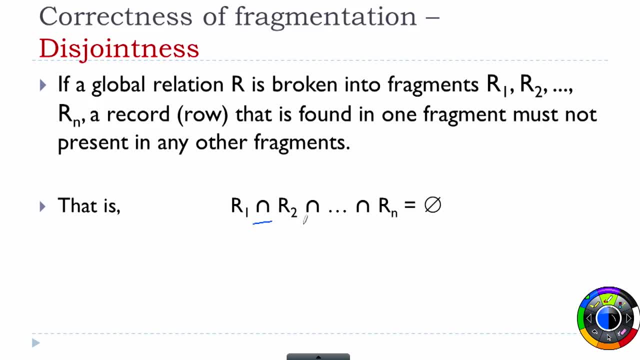 That means I perform an operation intersection between the records of all these sub relations and I must get null as a result. So no records should be common in more than one relations. That is the disjointness rule is all about. So when we have these three rules, completeness, 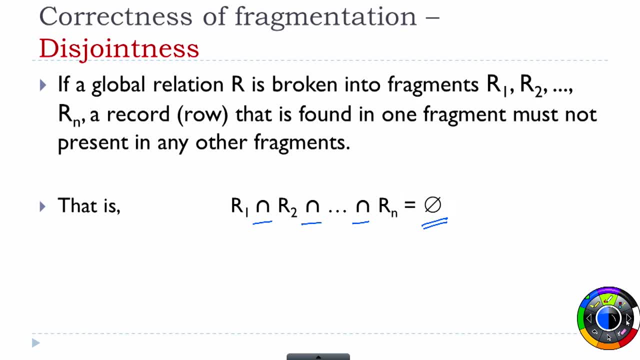 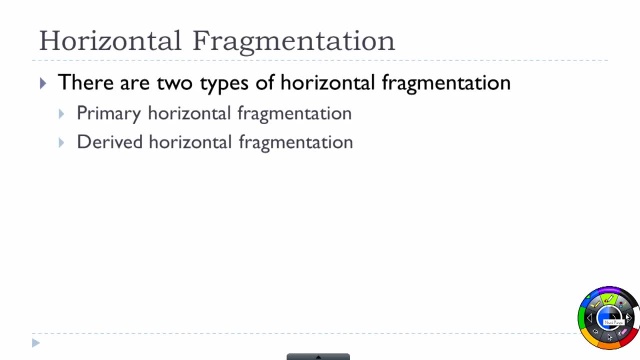 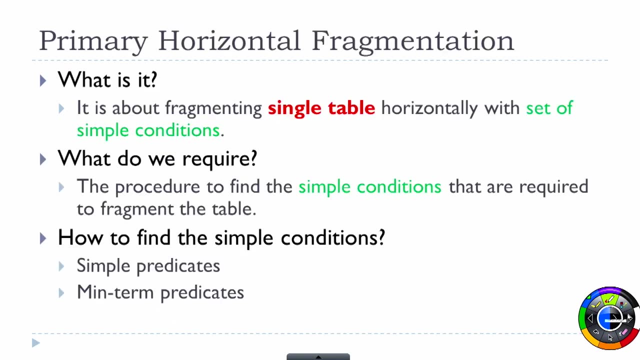 reconstruction and disjointness and we would say that our fragmentation is correct. Let us go to the next slide. So we have horizontal fragmentation Now. there are two types of horizontal fragmentation. One is primary horizontal fragmentation. the other one is derived horizontal fragmentation. 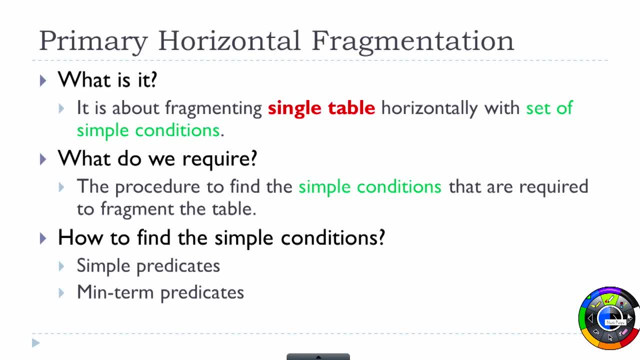 What is primary horizontal fragmentation? So very simple: it is about fragmenting a single table horizontally with a set of simple conditions. So what did I do For student relation? we have taken a global relation, student and we have applied the condition. 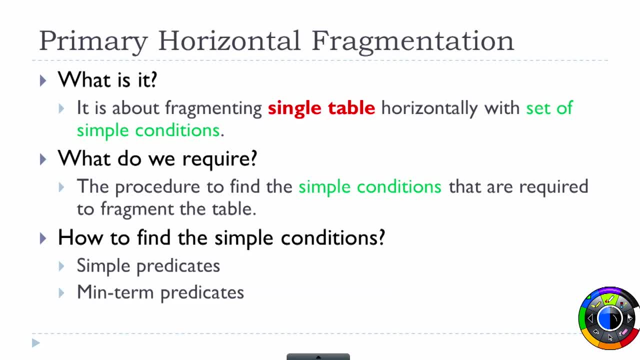 campus is equal to Chennai. another condition: campus is equal to Vellore, campus is equal to Mumbai, and so on. So now what happens is, what is the result I will get is my horizontal fragmentation, which is primary horizontal fragmentation. So it is about fragmenting. 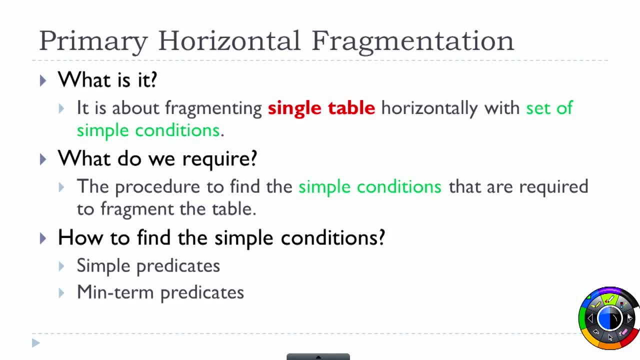 single table horizontally, with set of simple conditions. So now, what do we need for achieving this? So, we need to find the simple conditions that are required to fragment the table. So what is the result I will get? So what we 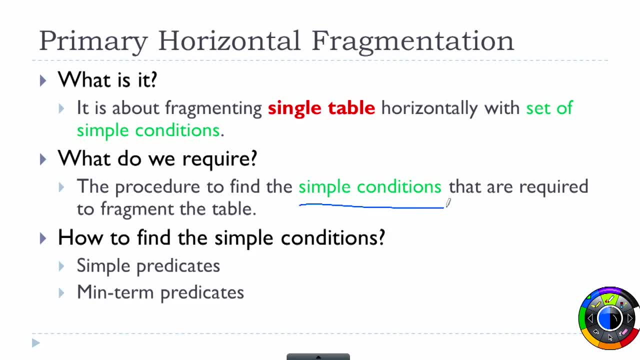 the table. Actually, it is the important problem to find these simple conditions. To find these simple conditions, what do we require is one is simple predicates, the other one is min term predicates. Before that, actually, what do we need is an application or set of applications. 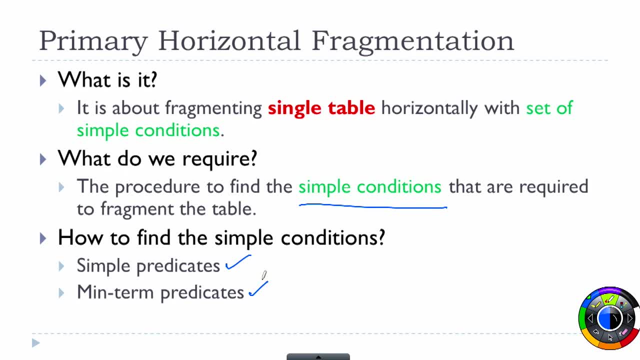 that are going to access these fragments differently. So that is a very important concept, So that we need to identify, as a designer, So what data are going to be placed where and all the applications that tries to access this particular data are able to access the. 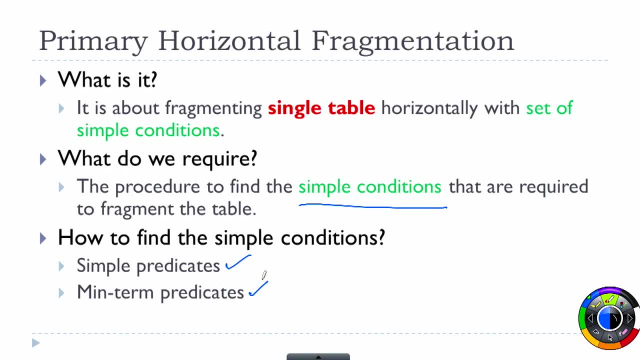 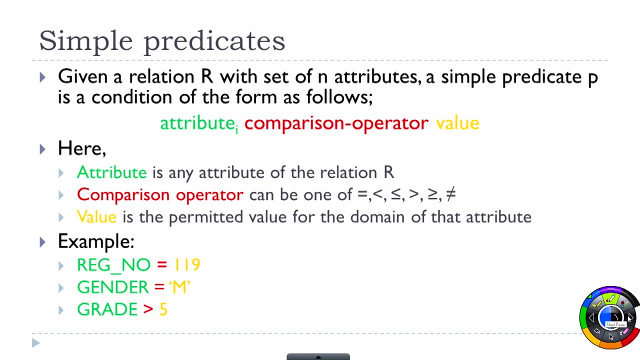 data, locally or not. So these are the concepts, the background concepts that we need before going to the finding this. that is, according to these conditions, we are going to choose the simple predicates and min term predicates. So let us discuss about simple predicates. So simple predicate is a simple condition. 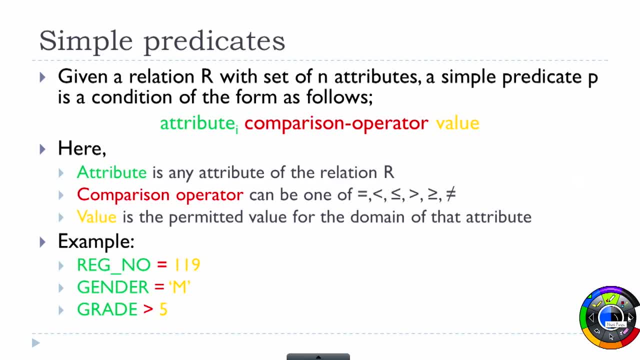 it is a condition. Example is: we have given campus is equal to Chennai. it is one simple condition. So, given a relation R with a set of attributes, n attributes, a simple predicate. P is a condition of the form as follows: So what do we have? An attribute is given there. 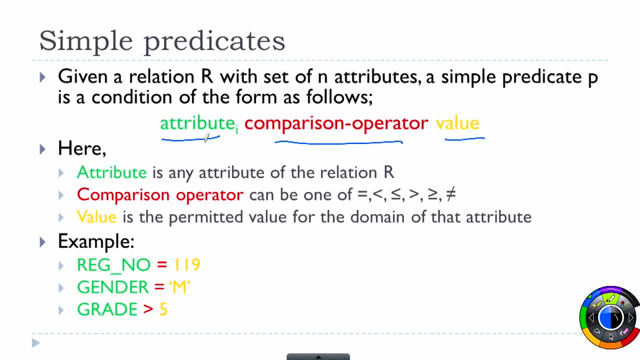 is a comparison operator and a value, So attribute is attribute i, so any one attribute, So attribute is any attribute of the relation R and comparison attribute can be one of equal to less than less than, or equal to greater than greater than, or equal to and not equal to. So these are all the condition comparison. 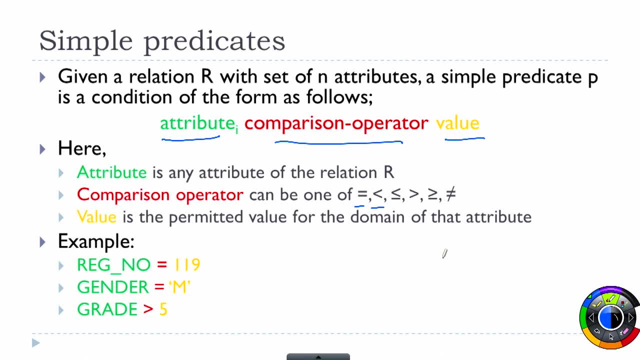 operator that we are using in writing SQL queries. while we put conditions in SQL queries, the same set of comparison operator And value is permitted. value for the domain of the attribute, that is, the values taken from the table line. So that is the domain of the attribute. So 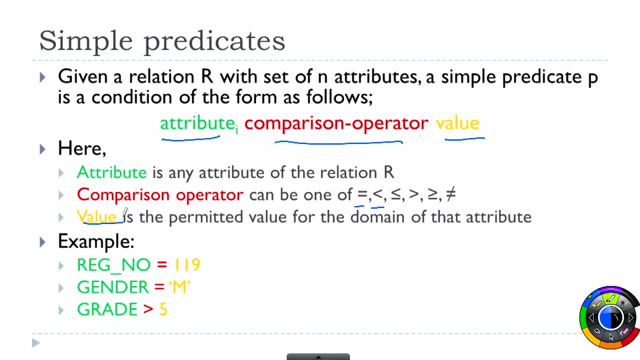 this value is the domain of the attribute. So, for example, if I say Chennai- sorry, campus- is equal to Chennai. So what is Chennai? Chennai is one of the permitted value for the domain of campus attribute. Chennai is one of the permitted values for the domain. 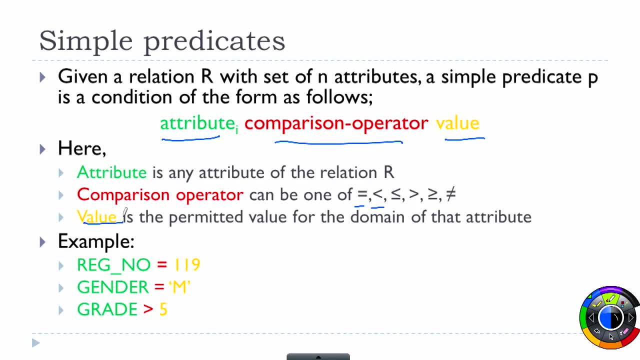 of the attribute campus. So that is the values taken. So examples we see here: register number equal to 119 is one of the one condition, one simple predicate: Gender is equal to male. that is another simple predicate. grade is greater than 5, that is another simple predicate. 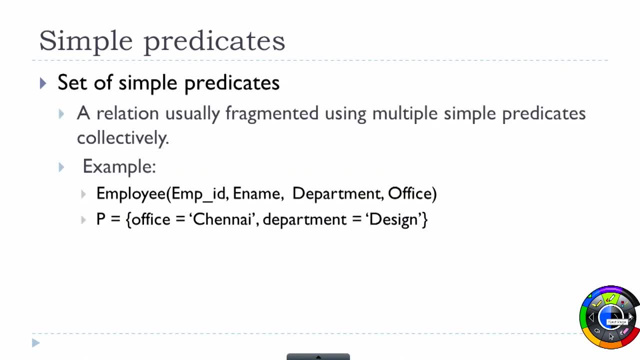 Now what do we need? is we? our application may tries to access the data differently in different locations, and not only one application is going to access all these data at all locations, So there are possibilities that multiple data or multiple locations, multiple applications. 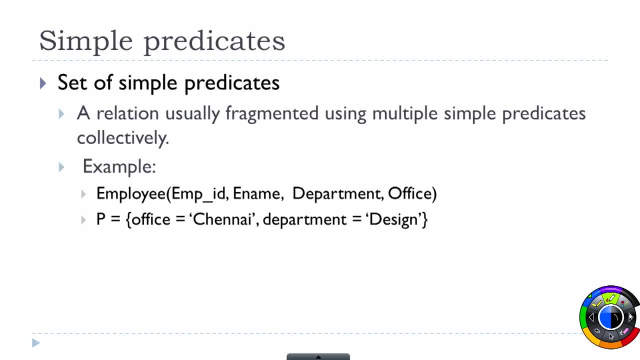 are going to access those data. So it involves definitely more than one conditions in most of these cases. So set of simple predicates is a collection of set of simple predicates and it is represented using P equal to as a set. So let us take 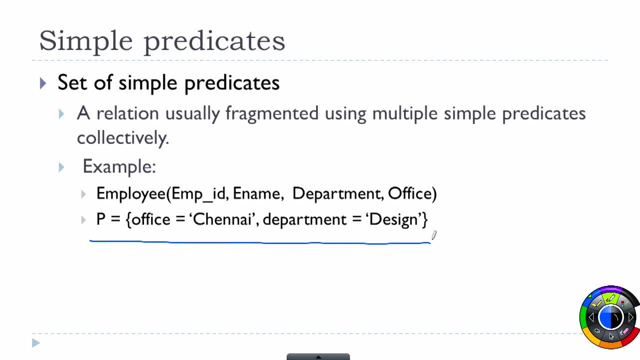 an example: employee table with employee ID, employee name, department and office as the attributes. Now I want to break my table. I want to break my employee table based on the office location, Chennai, and the department design, So I want to make this as one of the fragments. 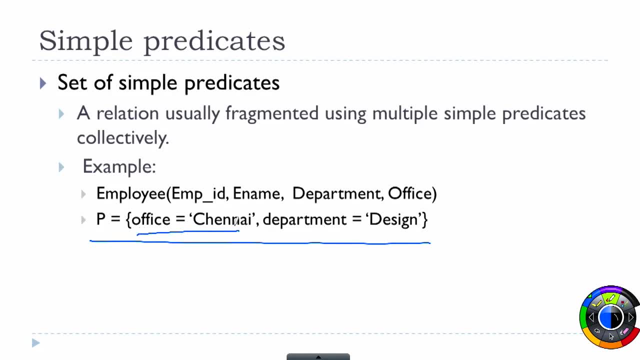 or I may have one simple predicate: office is equal to Chennai. that is, I want to fragment my relation with respect to this condition. Also, I want to fragment my relation with respect to this condition. So these two conditions may be connected or not connected. the difference, But what? 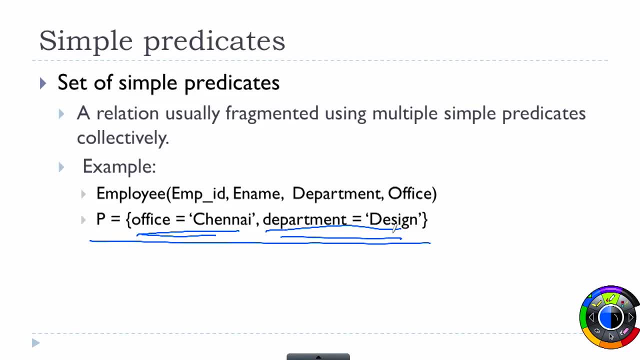 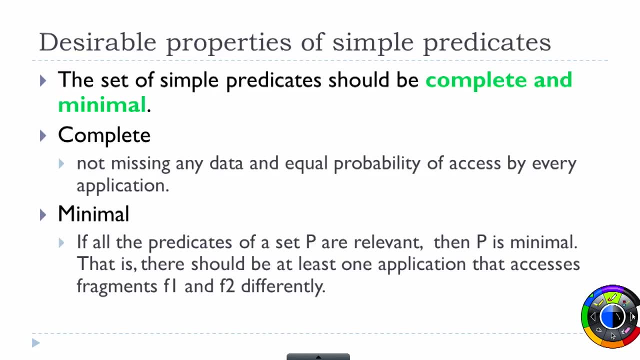 we have is we have two simple predicates, So my set of simple predicates have two different set of two different simple predicates. Now, when I take simple predicates, can I just like that, choose the set of predicates? No, the set of simple predicates should be complete. 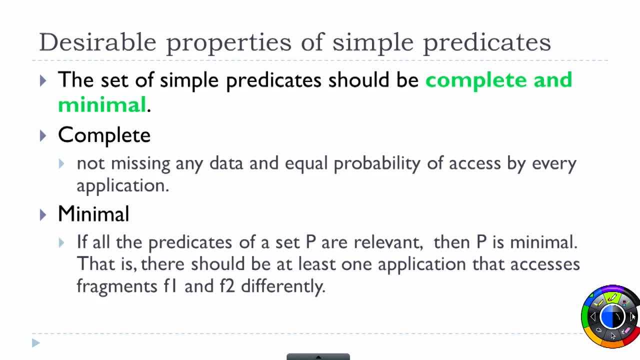 and minimal. Complete and minimal. So the set of predicates should be complete and minimal. Complete and minimal means complete, means not missing any data and equal probability of access by every application. So we do not want to miss any data. So when I apply, 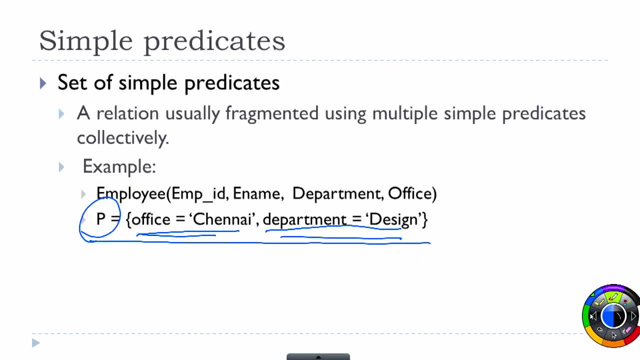 this condition. what will happen? For example, let us take this condition: office is equal to Chennai. Now, where, when there is Chennai, only one office? So what is the purpose of fragmenting this relation? Absolutely not So. that means. what is the purpose of fragmenting this relation? Absolutely not So. that means: 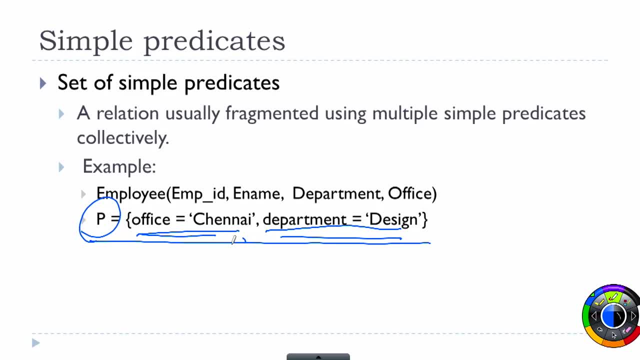 office is Chennai. I want to fragment this relation, but there are other offices as well. that is the meaning. So when I put the condition office is equal to Chennai alone, it is not going to give me the result. Suppose I have four different offices. Now what are my simple 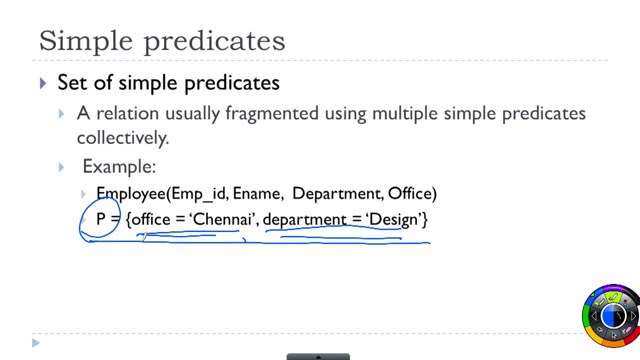 predicates are: Office is equal to Chennai, office is equal to Mumbai, office is equal to Delhi, and so on, But instead, in other words, I can simply represent this one as office is equal to Chennai And another condition is office is not Chennai. So I am going to 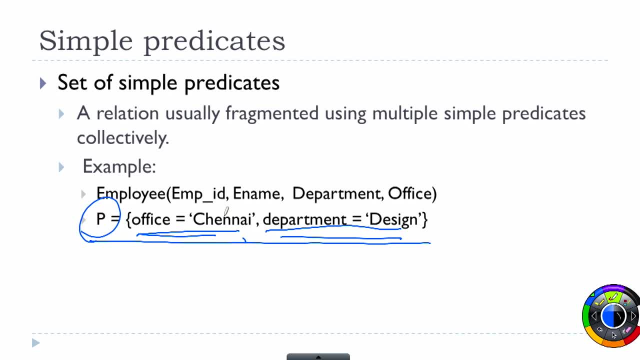 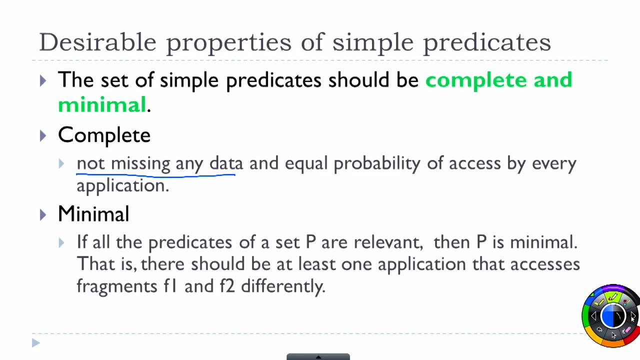 say, office is not equal to Chennai, Now that will include all the other offices, all the other offices into this particular condition. So that is what we need. So this is says it is complete. I am not going to miss any data. I am not going to miss any data and 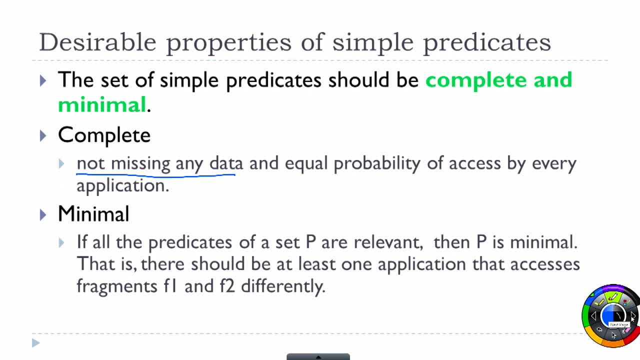 equal probability of access by every application. Every application tries to access this particular data is having equal probability. That means all these sites. why I am breaking my table, why I am placing my data, why I am breaking my data, why I am breaking my data, why I. 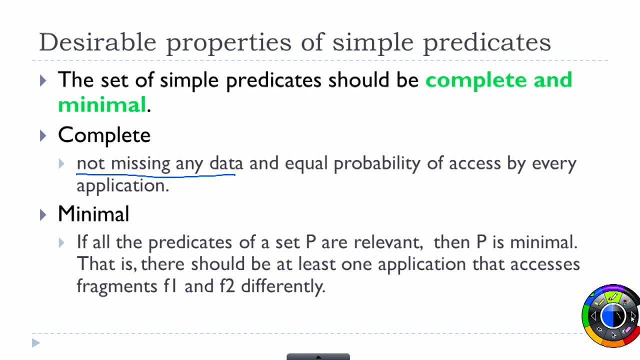 am breaking my data in different locations. all it is all. have some amount of equal probability. The second property: minimal. If all the predicates of set P are relevant, then P is minimal. There is. there should be at least one application that accesses fragments F1 and F2 differently. 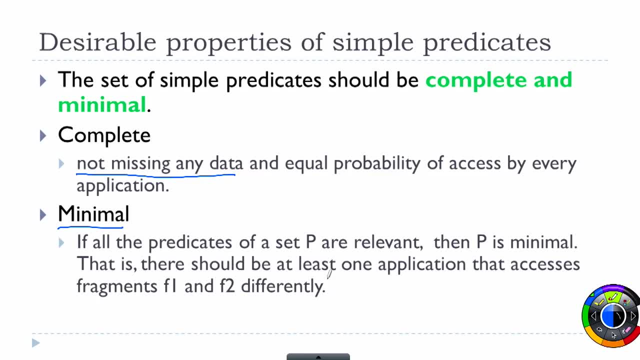 So why I want to fragment F1 and F2?? Why I want to fragment F, that is, relation R into fragment 1 and fragment 2? Because there are two applications. So I want to fragment F1, fragment 2, because there are some applications that access fragment 1 alone. There are some. 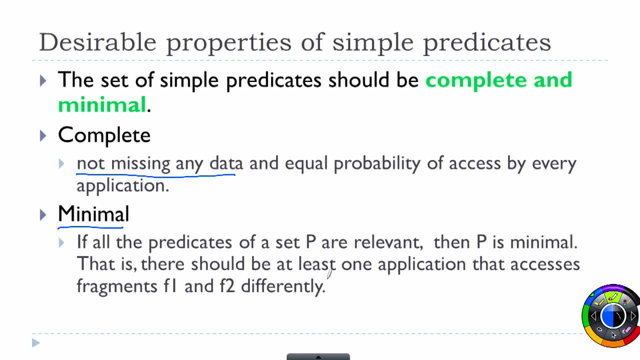 applications that access only fragment 2 alone. So that distinction I want to give, So that if all the predicates of set P are relevant, then P is automatically minimal. So I should not include unnecessary fragments with by introducing some other simple predicates. 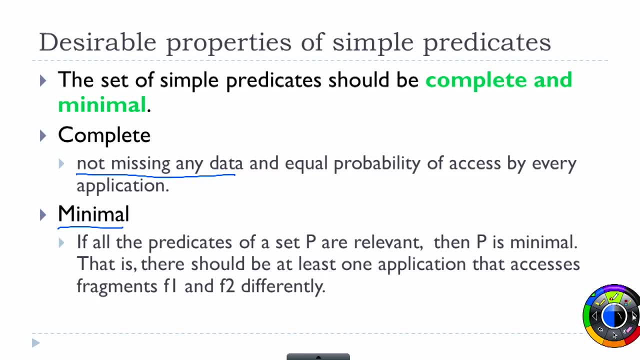 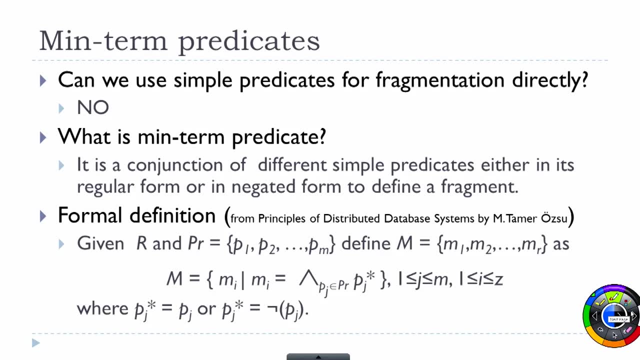 That is what the minimal property, minimal property- is about. So next one I am going to read: So the next one is min term predicate. So can we use simple predicates for fragmentation directly? The answer is no. That means I cannot use individual simple predicates on each relation to fragment this. 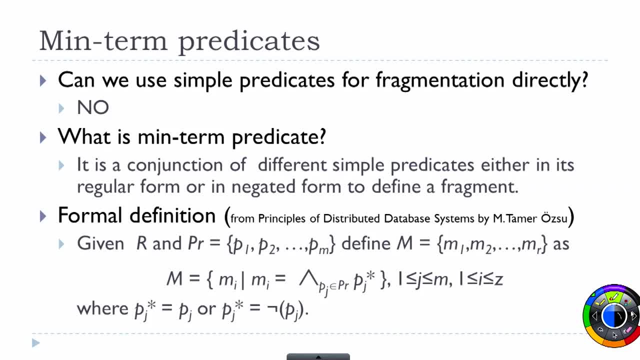 relation, so that tribal result may end up in replication or result may end up in redundant data. So what is min term predicate? So conjunction of different simple predicates, either in its regular form or in a negated form, to dependent predicates. So this is: 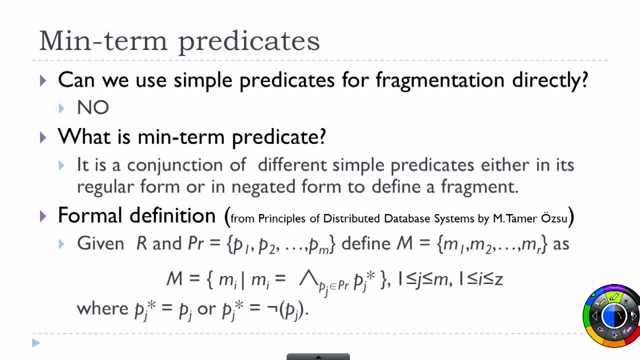 the min term predicate set P, So we can use min term predicates for fragmentation, only define fragment. So what we do is: given relation R and set of simple predicates P1, P2 and so on. Pn: we can define min term predicate M equal to M1, M2, M and so on. M R as the 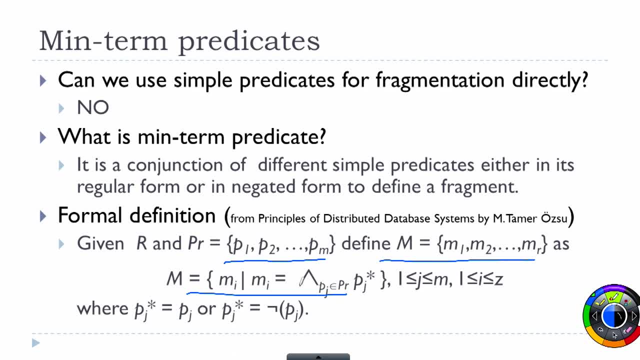 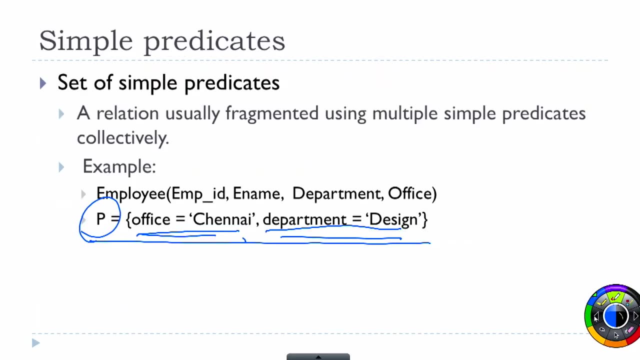 conjunction of the conjunction of, that is, this is conjunction of all simple predicates, in its original form or in negated form. that is what we want to have. So suppose, if I say, in this employee table office is equal to Chennai. So I want to. 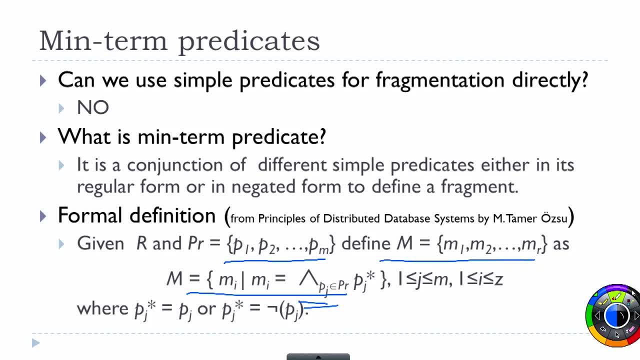 include other offices as well, but I do not want to create separate fragments for each of my offices, So I want to create only for office Chennai, and other offices automatically goes to the another fragment. So what is the condition is required? That is my first simple predicate is: office equal to Chennai is one fragment, So automatically. 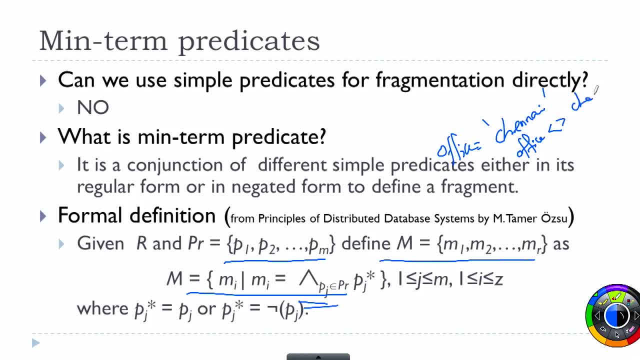 I have to include: office is not equal to Chennai, So that will end up in a separate, different fragment. So that fragment is another fragment. That is the min term predicate derivation. So I am going to include: either I am using the regular form or in a negative form. So simply I can put in other words: 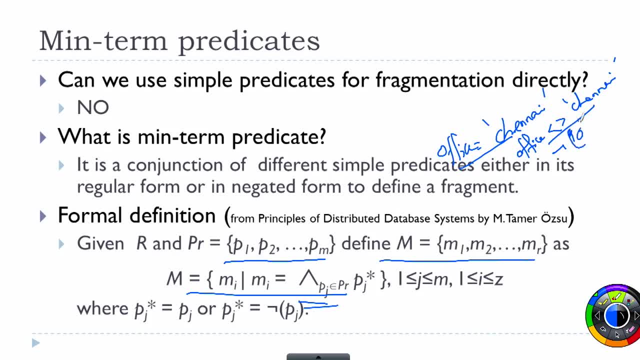 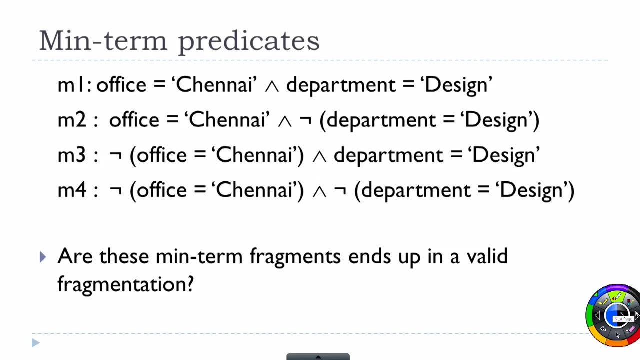 I can put negate of office equal to Chennai. This way also, I can represent this. So what will I get for our set of simple predicates of office equal to Chennai and department design without any further simple predicates Now, by applying this min term fragmentation? 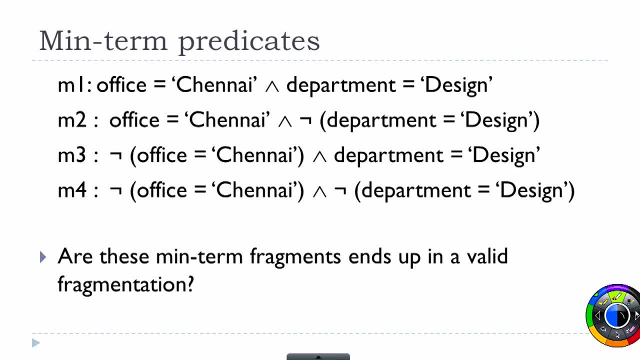 rule, we will get 4 fragments, 4 min term predicates: M 1, M 2, M 3 and M 4.. So what is M 1?? M 1 is office is equal to Chennai and department equal to design. because I do not. 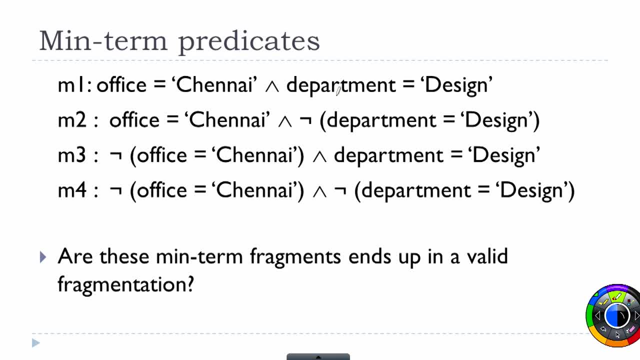 want to use R in between. So when I fragment my relation I want to use- I want to follow this- correctness rules. So once I fragmented my relation, the result should be obeying that completeness correctness rules. So for that one I cannot use these rules. So I 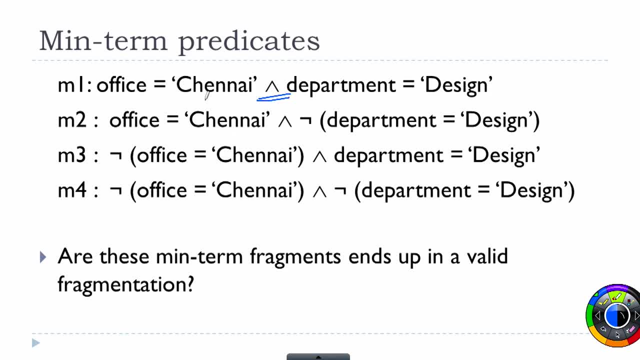 this R as a symbol, because R will include office is Chennai, all records that satisfy this condition, and separately. department is a design. If department is a design, either department design or office is Chennai, all the records will be included in this fragment. So that is wrong. 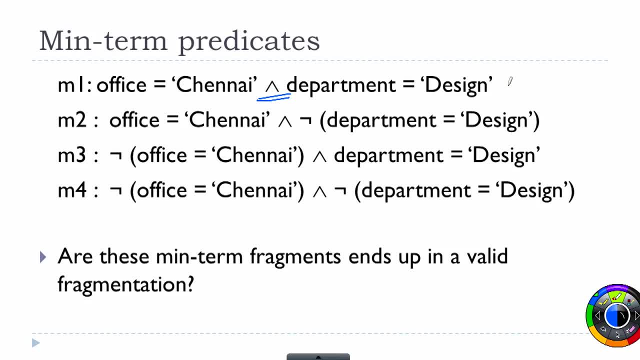 So you will get finally disjointness property violated. So to avoid this, what we do is only we use conjunction between multiple conditions. So we have here only two simple predicates. So we connect these two simple predicates using conjunction and 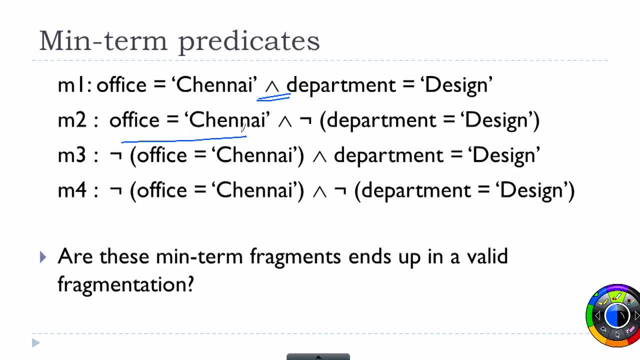 Now, second condition is office in its original form, office equal to Chennai and department other than design. department other than design, So negate of department equal to design. And third min term predicate: office is not equal to Chennai, So we negate that office is not equal. 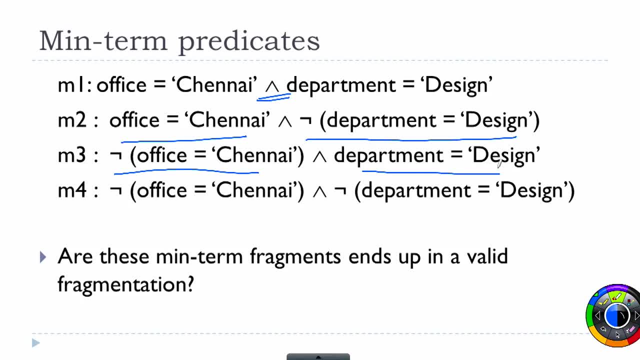 to Chennai and department is design design department, but office is not in Chennai. And the fourth one, office is not equal to Chennai, as well as department is not equal to design. So what will happen is this will first min term predicate will accept all the records. 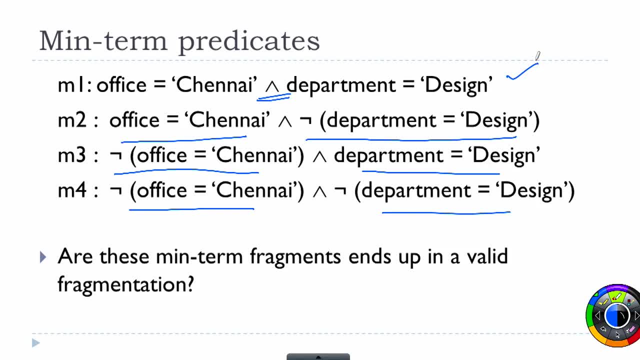 where office is Chennai as well as department is design. The second record will include all the other departments that has office in Chennai. Third min term predicate will include office other than Chennai and department is design. The fourth one will include all the other records, all the other. 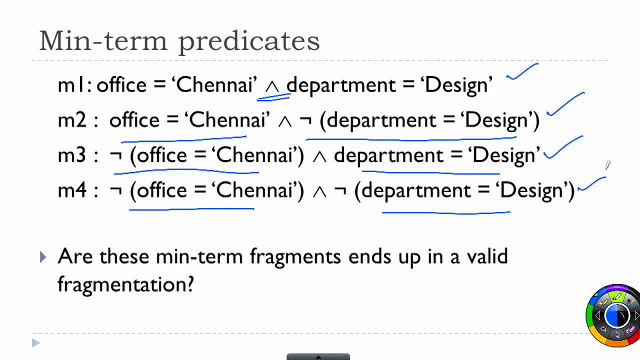 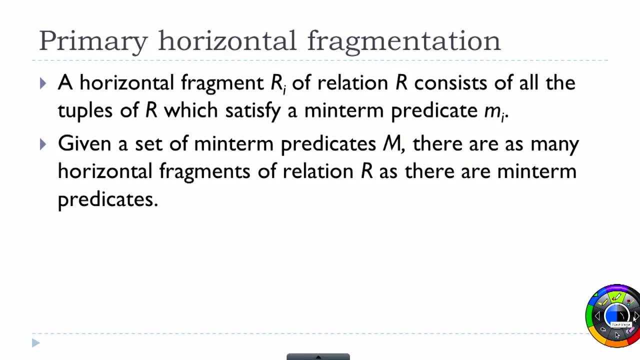 records. Now the question is: are these min term fragments ends in a valid fragmentation? That is a question. So how do we check that? So, primary horizontal fragmentation: the horizontal fragment Ri of relation R consists of all the tuples of R which satisfy the min term. 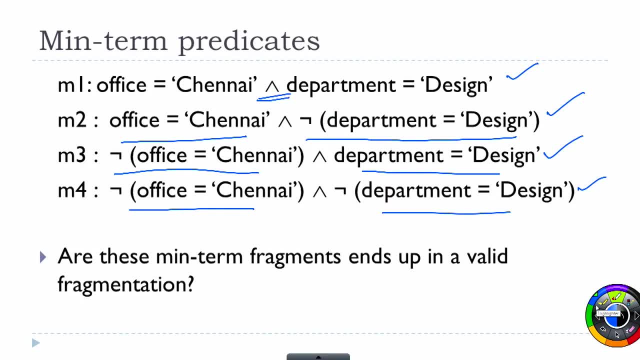 predicate Mi. So what we do- All these min term fragments- ends up in a valid fragmentation. So we are going to use these min term fragments- min term predicates- to write a query so that I can filter my data from a original table. So, given set of min term predicates. 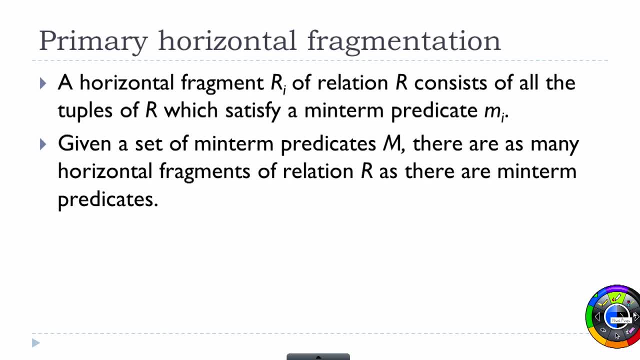 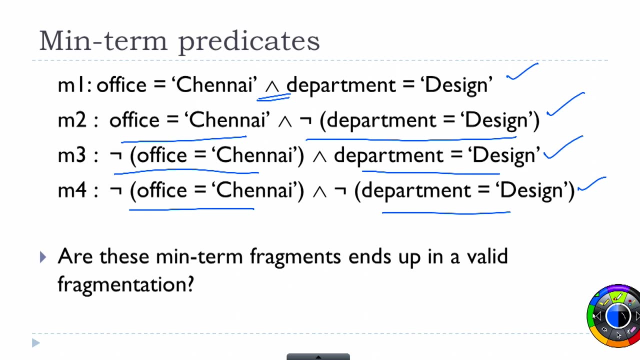 there are as many horizontal fragments of relation R as there are min term predicates. So if I am arrived at 4 valid min term predicates, that means I am going to break my original relation R into 4 fragments. So that is a result of this one. So what I derived is: I found 4 valid min term. 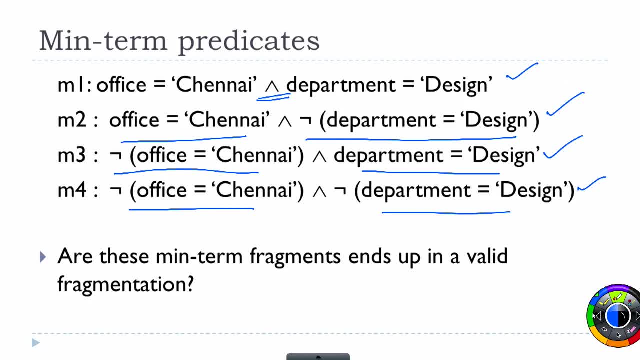 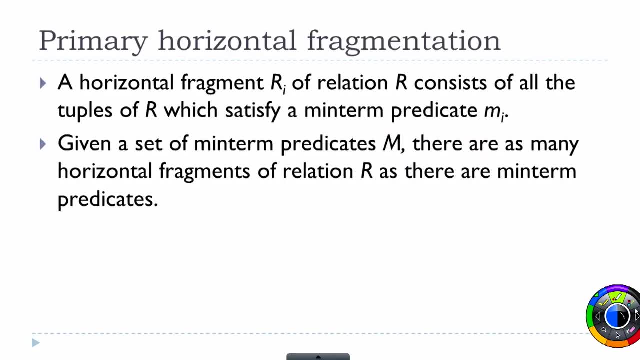 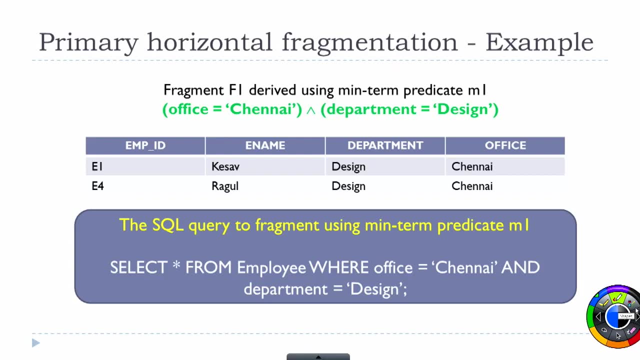 fragments of min term predicates, of derived 4 min term predicates from the set of simple predicates and I am going to apply these to derive sub fragments, the sub relations. So let us discuss this with a relation example: employee. So fragmentation, primary horizontal fragmentation example: See here. I have a table from that table. 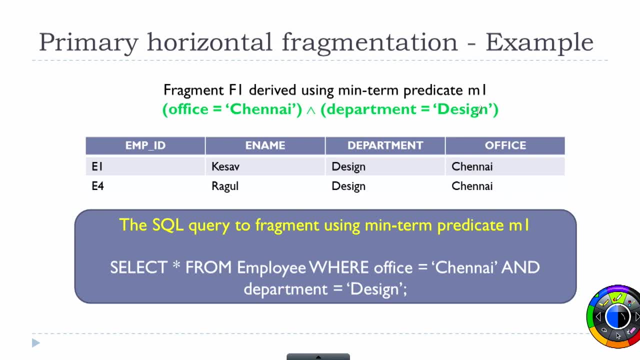 my condition says: office equal to Chennai, a department equal to design, and what I arrived at is some records. that satisfies this condition. office is equal to Chennai and department is equal to design, So both should be valid. So I have used this query, that is, if I, if my min term. 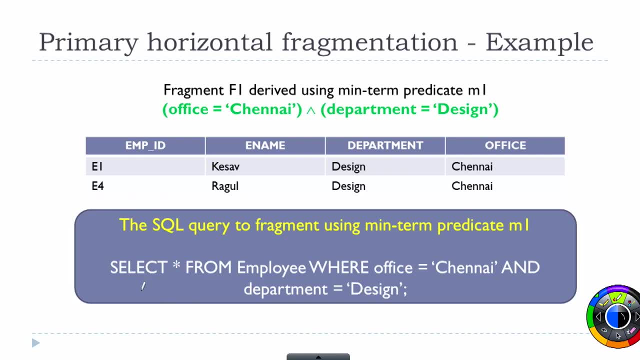 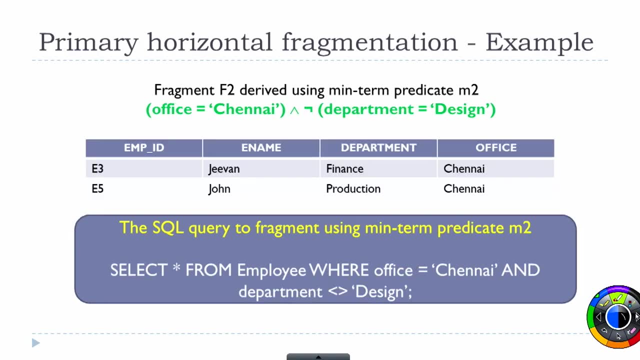 fragment is this? then I can derive the fragment one using the query select star from employee, where office equal to Chennai and department equal to design. Likewise, for the second fragment, fragment 2, is derived using min term predicate M2.. So M2, what does it say? Office is Chennai. 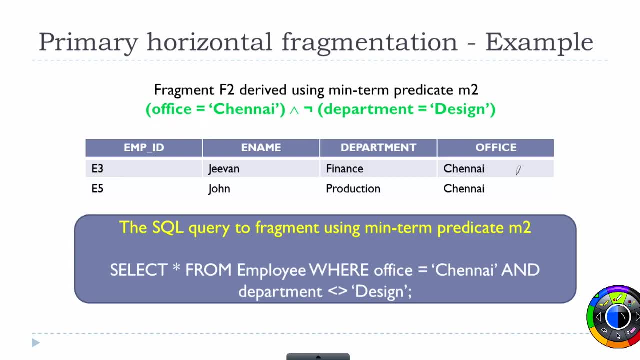 but department is not equal to design. So see here the example result: we have office, both offices: Chennai, that is office- attribute can accept only Chennai and department could be anything else other than design. It is finance and production, It is all finance and production. It is. 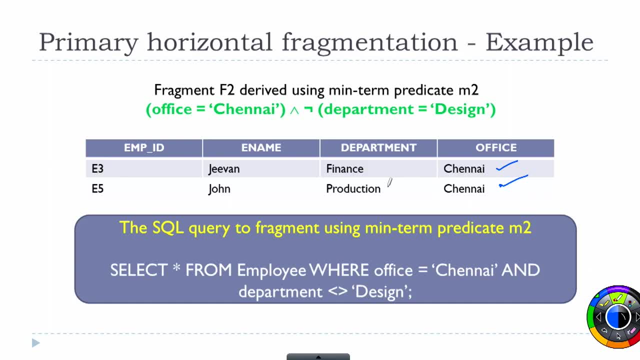 other than design. we have two different. any, any other, any other values. Again, the same min term. predicate M2 could be used to write a query in the var class select star from employee where office equal to Chennai and department not equal to design. it will end up in this rule implementing. 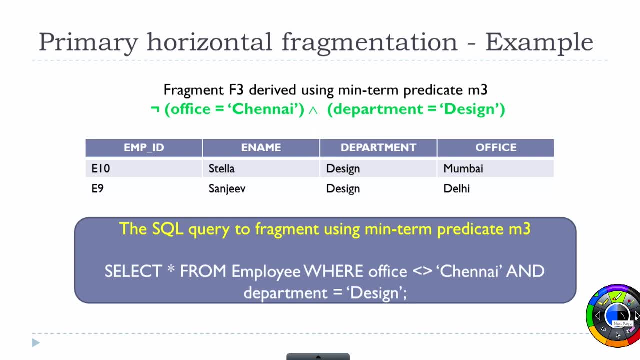 this min term predicate And fragment 3 derived using min term predicate M3, where office not equal to Chennai- See here- the result is Mumbai and Delhi not equal to Chennai. So the result is Chennai department equal to design. So all the department attribute value will be only design. 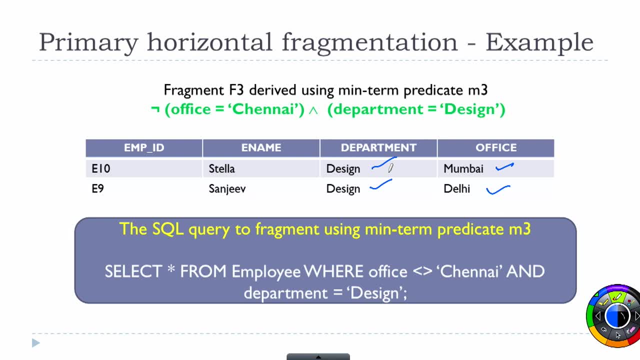 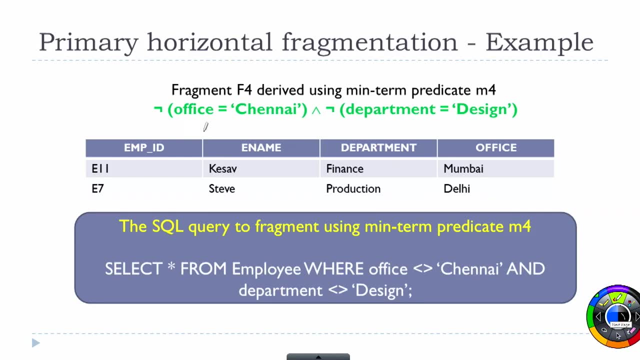 And this is a SQL query that can filter the data according to these conditions. And one more fragment: F4, where office not equal to Chennai, as well as department is not equal to design. So here, office is not Chennai, department is not design. 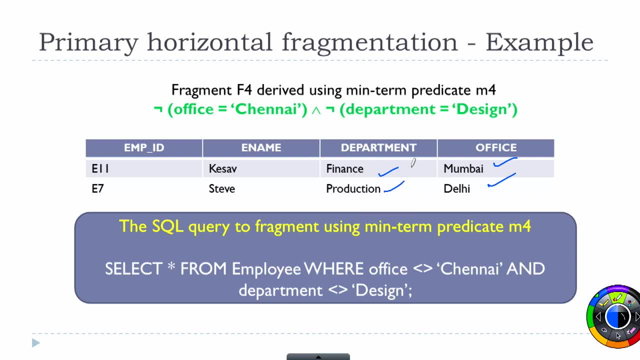 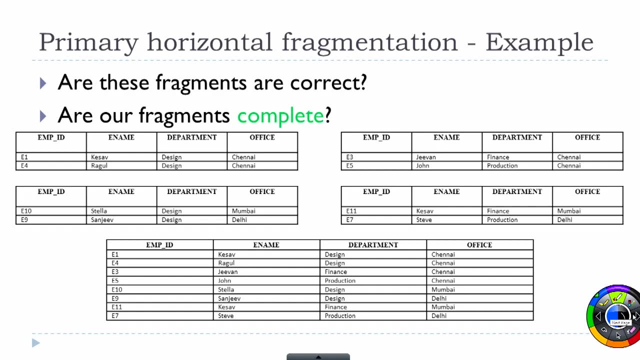 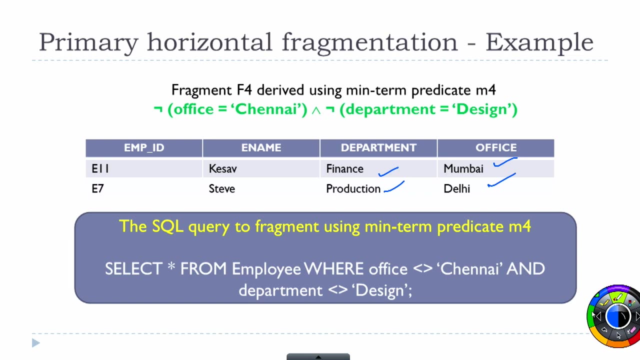 this is a result. So- and this is a query we can use to fight- filter the data from the original employee relation. Now we have fragmented our relation employee using four min term predicates, So these four conditions have resulted in four different fragments: Fragment 1, fragment 2, fragment 3. 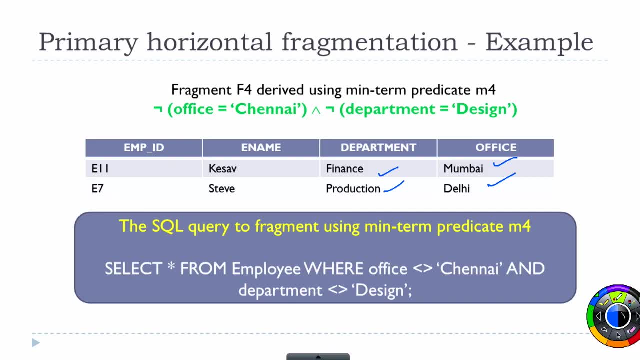 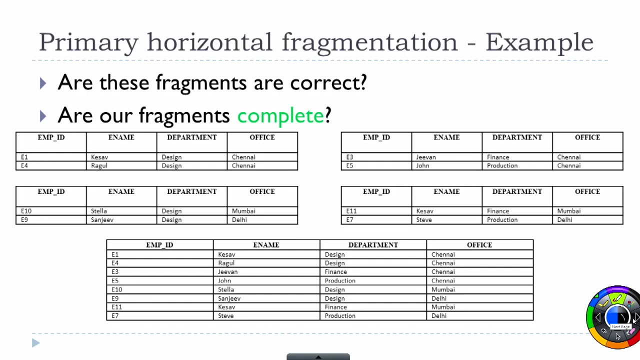 and 4, we have fragmented. Now the next important thing is the correctness rule. Have we fragmented our relation correctly or not? That is the question. So how do we ensure That we have to test these fragments against the correctness rule? So first one is: 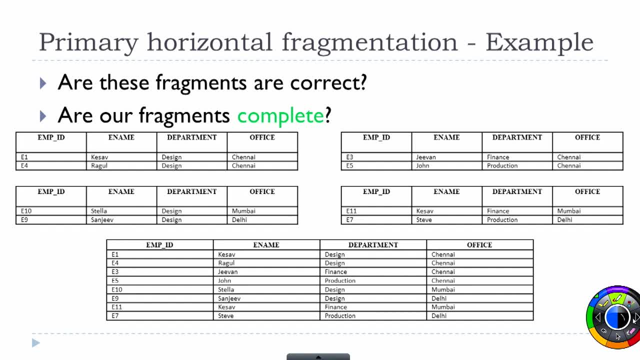 are our fragments complete? So what is complete? These records of the original relation R should be present in any one of these sub-relations: R1,, R2,, R3 and R4.. So we want to ensure that no records from the original relation is missed. 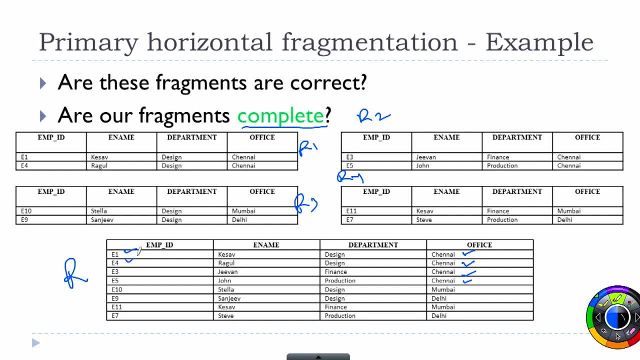 See here: the first record, E1 and E4, goes to relation R1, sub-relation R1.. Second, E3, E5, these records are going to R2.. E10, E9 ends up in sub-relation R3.. And finally, 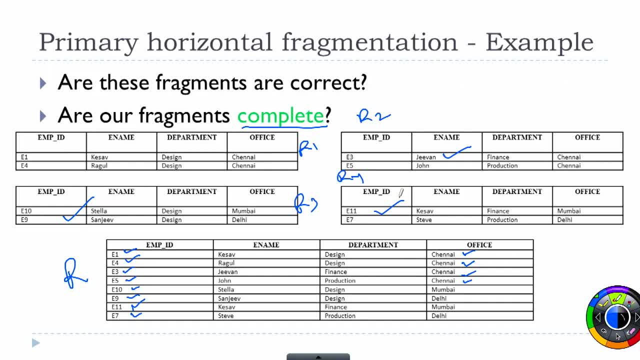 E7 ends up in E7 ends up in R3.. So we have totally eight records in this original relation, R employee And all these records are fragmented and ends up in different sub-relations and no record is missed. So that means our fragments are complete. So we can say that our fragments are. 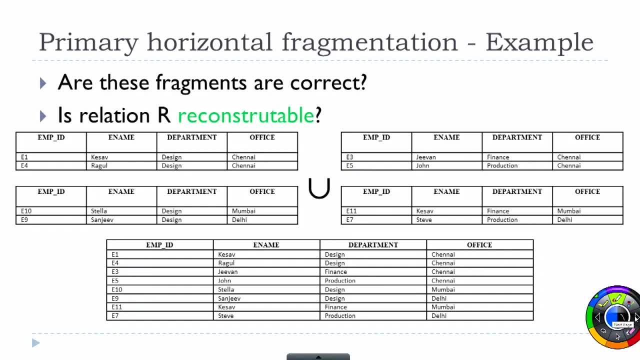 complete. Second problem Is a relation R reconstructable. Can I reconstruct? So the second property is about reconstruction. So can I reconstruct my original relation R from the subrelations, the fragments. So when I perform union between R1, R2, R3 and R4, we will get R back. So no records are missed, no changes happen. 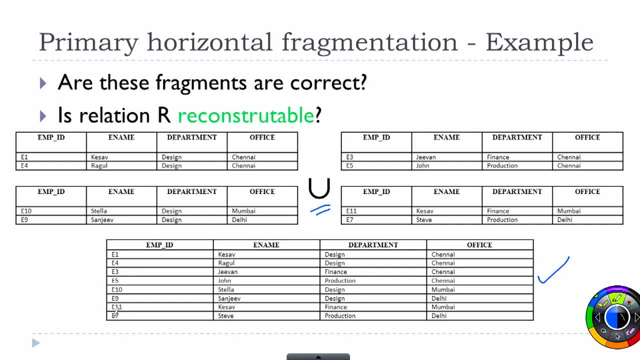 So this was my original relation. this is my original relation and this relation is no change. That is what the advantage is about. So I am not going to lose any data. So R is reconstructable from the fragments R1, R2, R3 and R4.. So this is second rule also. 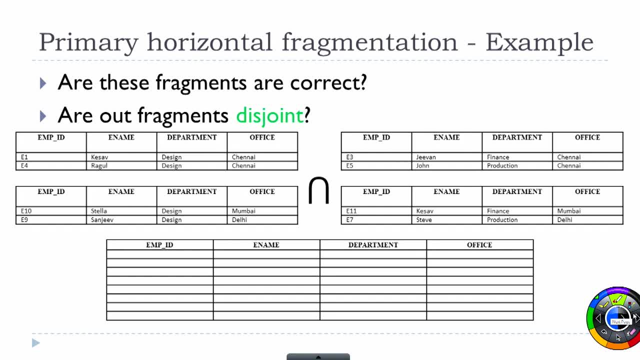 valid. So third rule. So third rule is about disjoint, So no record should be common between these different fragments. That means if I perform R1 into R2, R3, R4, R5,, R6,, R7,, R8, R9, R10,.